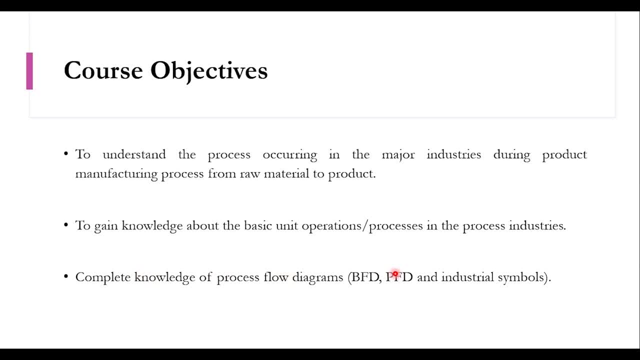 and unit process deal with the chemical processes and complete knowledge of process flow diagram, which is PFD, BFD and industrial symbols. PFD stands for Block Flow Diagram, PFD standards for process flow diagrams. So the books which are recommended for this is: 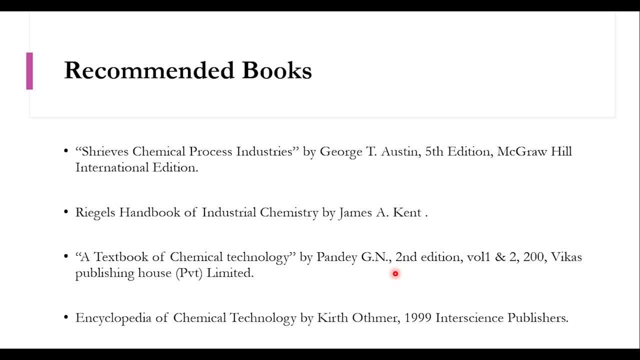 Sharif's Chemical Process Industries, Rieger's Handbook of Industrial Chemistry, our textbook of chemical technology and Encyclopedia of Chemical Technology by Kirkh Uhtmar. What are the resources? and in this knowledge, would you like to know why we need chemical processes? 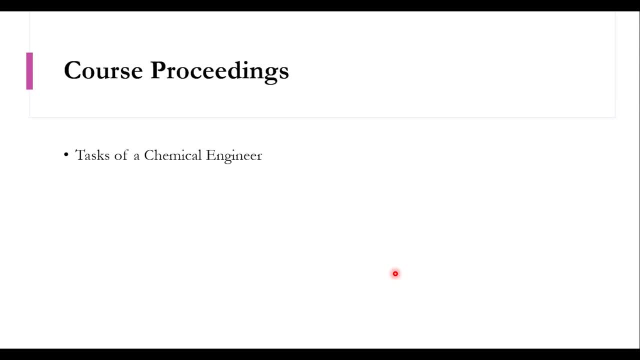 μ42,μg2,μ3,λº为- cishex Seal, lol-re incidence and offers for human beings with a certain behavior of chemical efficiency in industry. today's course proceedings number one is to first understand what are the tasks of a chemical. 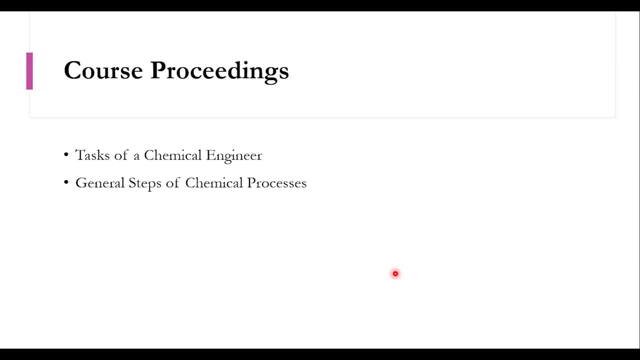 engineer. then the general steps which are included in chemical processes, industrial manufacturing process, chemical process design with its requirements, example of a process. so what are the tasks of a chemical engineer? obviously the chemical engineer have to do various tasks. it is called as an all-rounder among all engineers, so its number one task is to convert the innovation. 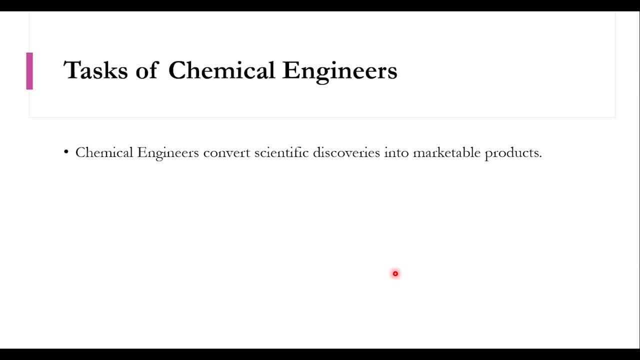 to a product because we have to sell the product. first. we get some innovation and then we have to translate into some product and obviously we have to design a process or a plan to make it happen. and obviously that include the research and design, the chemical production, construction and operation. 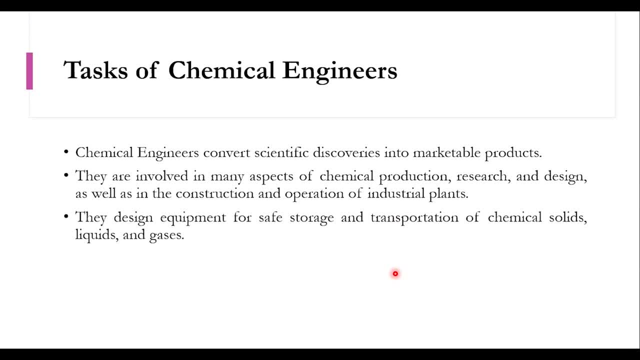 of industrial plants. then they design equipment for safe storage and handling and transportation of chemical solids, liquids and gases. then the control system, because obviously for a successful plant operation the control system should be perfect or adequate for it to run. so design control system for chemical plants based upon data from lab experiment and pile plant operations. and, last but not the least, 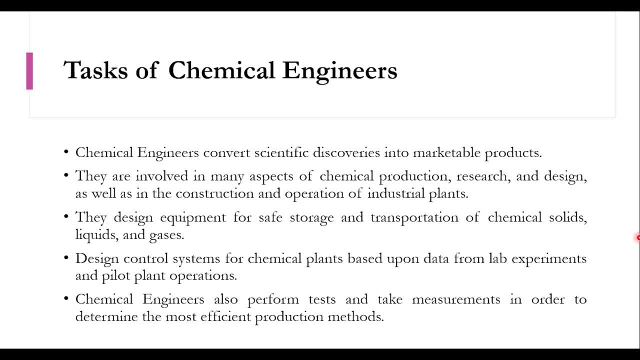 they also perform tests and take my years in order to determine the most efficient production methods. obviously the role of a chemical engineer to select the production technique which is the best possible technique among the various production techniques for the same product and then have to design the plant, have to erect the plant, commissioning installation operation and obviously have to 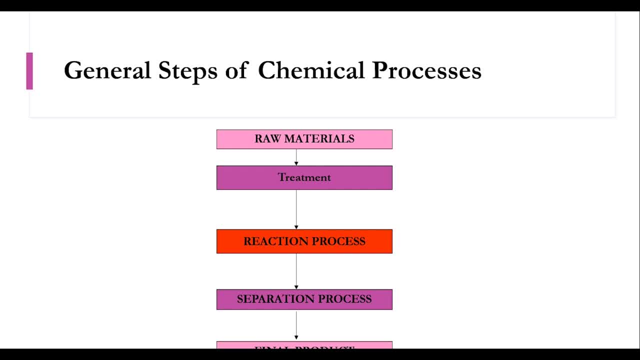 improve it as well. so, if we talk about it, the general manufacturing plants or the general steps, that starts with the raw material, the treatment process, the reaction process, the separation and the final product. if we divide the overall system이 that reactors of the reaction process is the core of our chemical plant. 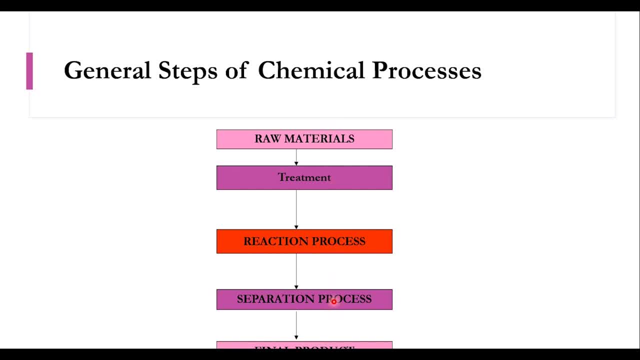 These are the pre treatment steps and these are the post treatment steps. the pre treatment steps include the raw material, that Patent like filtration, and so on, different techniques, then the reaction system, Then the Jerusalem, which includes Cyclone separator, and different techniques, distillation song, and then we get the final product. 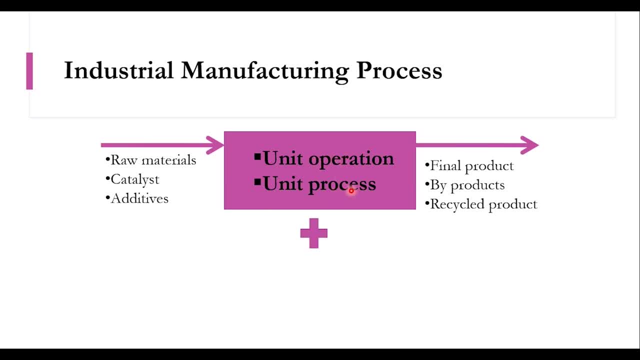 if we talk about the additional manufacturing process, obviously a- you you know- operation unit process or a combination of both may be required to convert raw materials into final products. it may include catalyst additives as well and the final product also accompanied with byproducts and recycled products as well. but this is not limited to this part only. it also 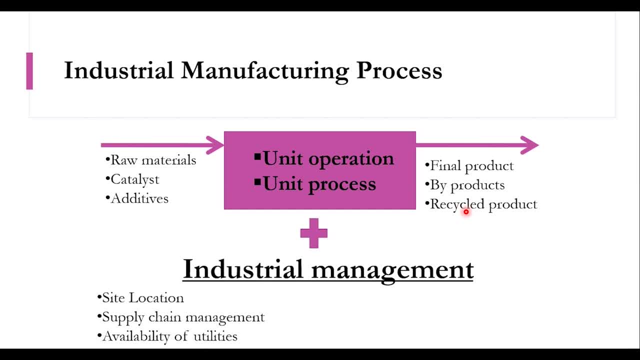 include the industrial management, which include site location, supply chain management, available of utilities and human resource management. you have to understand it that all the technical work is obviously going on here, but your task, once you are going to the industry, is to do the management process, and this management process is the fundamental, or i can say the core process. 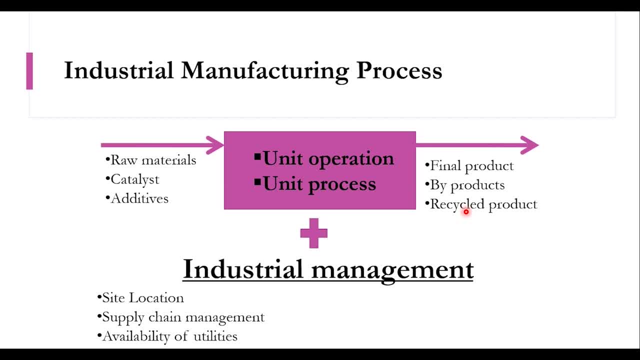 once you are operating a plant because technically you are strong, that is good. but if you are a bad manager, you don't have a place in that industry for so long. so obviously industrial management is also a key part: affluent disposal, climate, environment, local community consideration and political and strategic considerations. so all these aspects have to be taken into account. 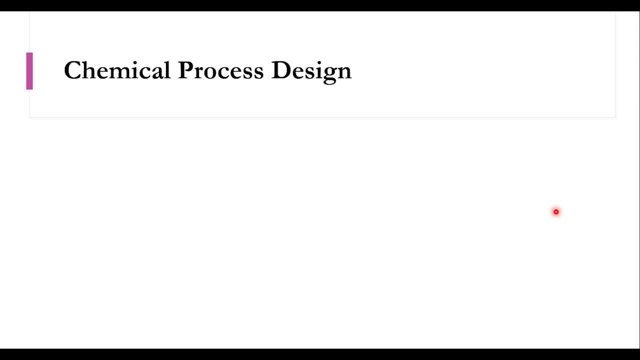 while going through an industrial manufacturing process. now, what are the requirements of a chemical process: design, the production rate, the capacity and the product which is required. how much purity is required? like you require 99 percent methanol or 99.5 percent methanol, obviously, even this 0.5. 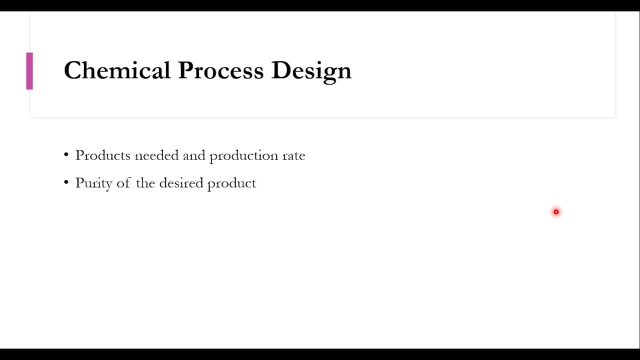 percent recovery or the 0.5 percent change can lead to different number of stages in the distillation process and so on. raw material to be used, obviously for different process or for different techniques. different raw materials could be used in the process. the available utilities: what utilities you? 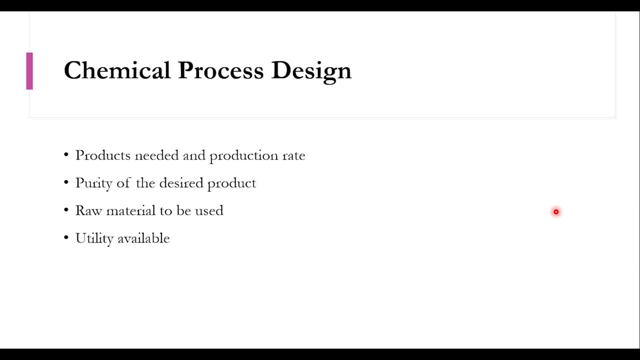 have? you have steam water chillers, chilling water and so on- what type of utilities you are having in the system? what will be the process route? that is how important because it will determine the raw material in the system, because for different routes the raw materials could be different in the process. 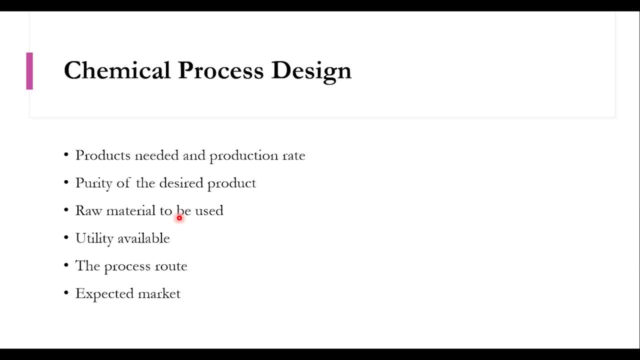 and so on. if you are have a device in the system where you are having to sell the product, you are having to sell the product. the process is going to be different. in the process- and most of the times it is some purpose- you will have a service which from this process, needs. 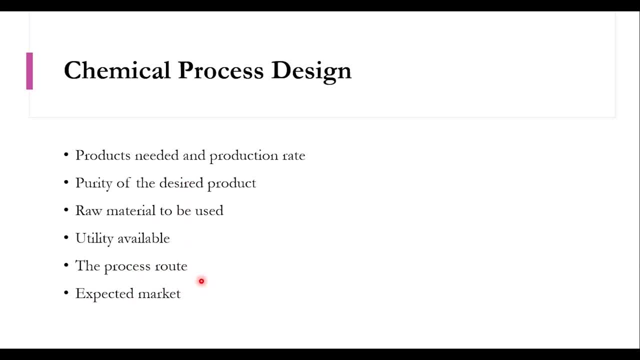 to prove it. the process route details are straight away where you have to throw battery connection the previous machines. we bring it through the system and promote this process to the customer so that he must come out with the new yogic ready to go lake tall and his 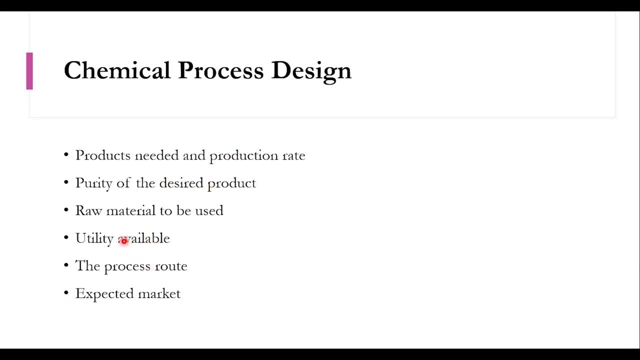 products. with this technology he becomes completely free from that need to be clear. the product will be consumed right away. then you have prepared the organic materials to use as a raw material. then you will come to the process route and utility available and obviously the site selection again place a new material is between 1 $ an hour if in that case you have no need to do. 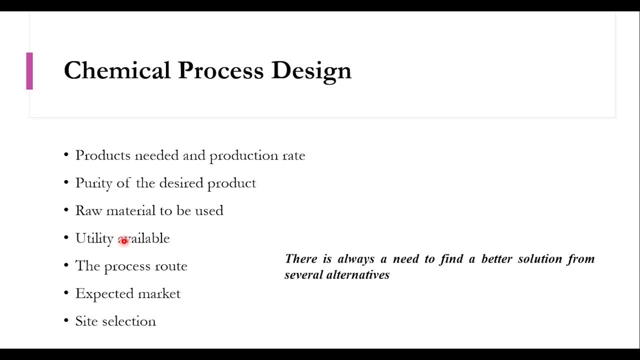 this. let us go to the second portion, and then we will get bit more Azerbaijan as well in the next vital role in it. however, this does not end there, and there is always a need to find a better solution from several alternatives. then again, process flow sheet, description, mass and energy. 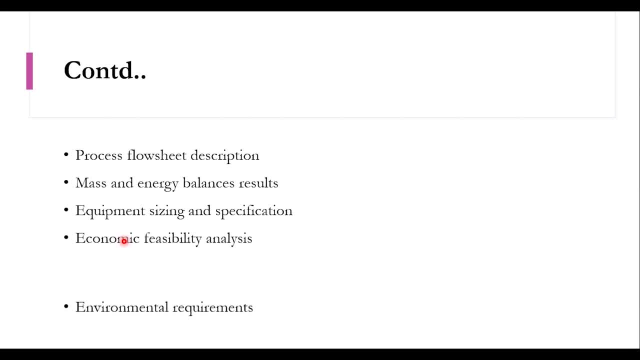 balances, result: equipment sizing and specification, economic feasibility analysis, environmental requirements and finally, the final report. obviously, if you have done your fy dp- the final year design project- or if you are new to the fy dp, you have to understand that you have to first select a process. or i can say: these all aspects are including in your fy dp. now, what you 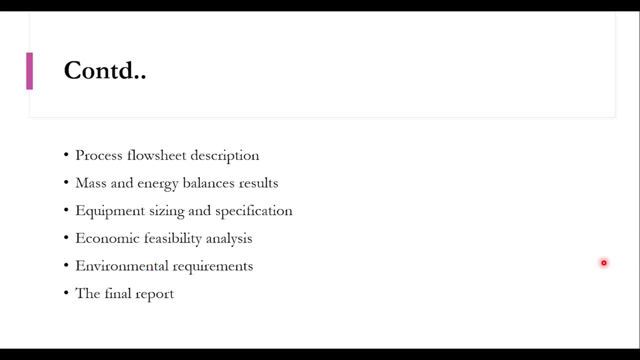 are doing in fy dp. obviously in an fy dp project you have to first select a title and that title is obviously based on the market requirements. then you have to select the production capacity and obviously it depends on the need of the country and particular facility. then you have to. 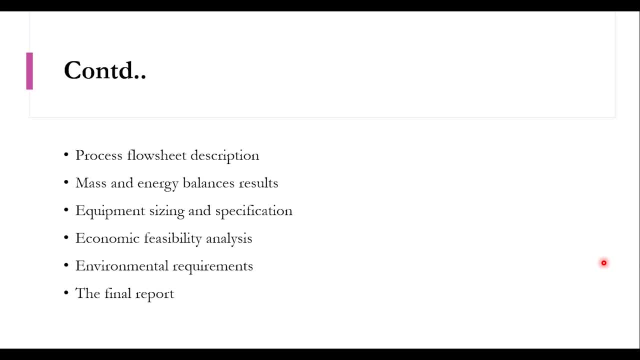 select the process, because to make the product there could be different process alternatives and you have to select the best of them, obviously based on different advantages, disadvantages and so on. then, once you have done this, you have to prepare the process flow sheet, or i can say process flow. 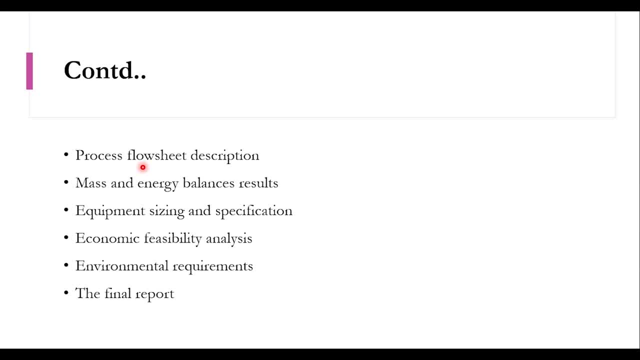 diagram of the system, and then you have to do the material balance, energy balance, costing, designing, so on, and all these aspects are covered in. so this is the overall process design you are doing, and again it includes various plant design aspects like the site selection, the mechanical design of the equipment and